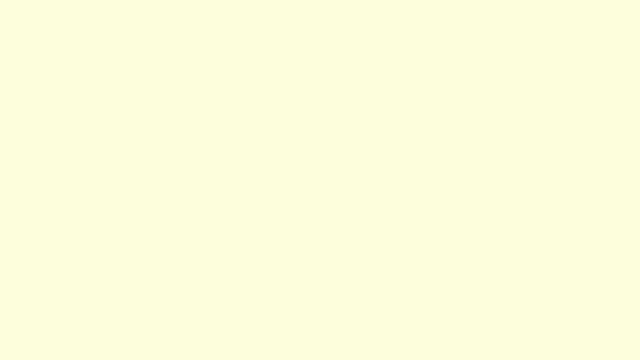 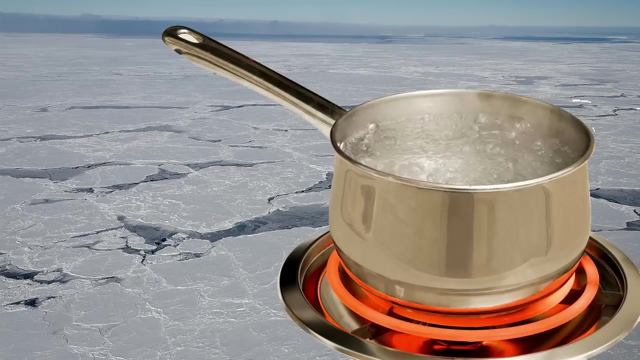 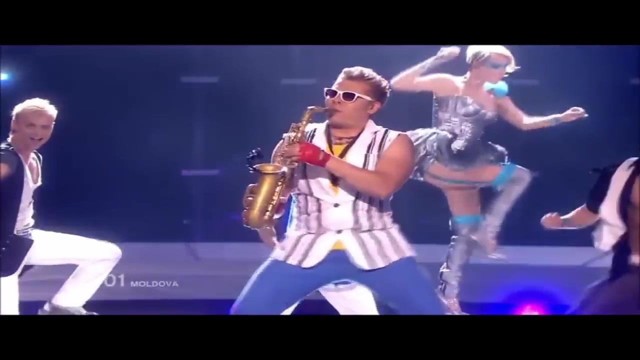 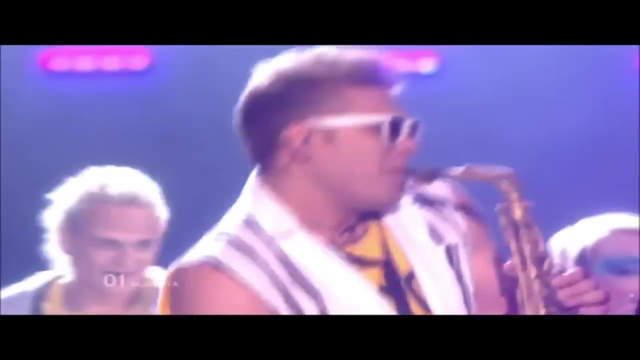 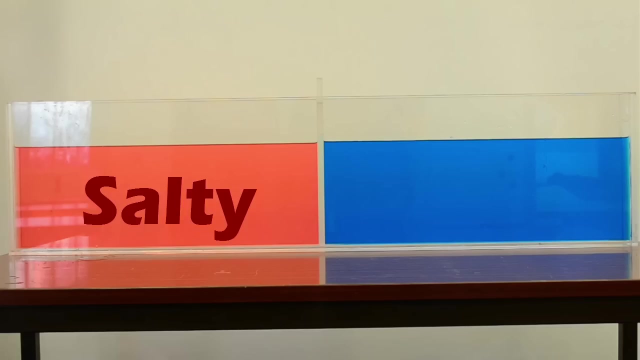 iceberg melting and river runoff makes the seawater lighter. On the other hand, water cooling, ice freezing and evaporation make the seawater denser. Now watch this amazing video. Ok, getting back to our video, In this experiment, we used salt water on the left side and fresh water on the right side. 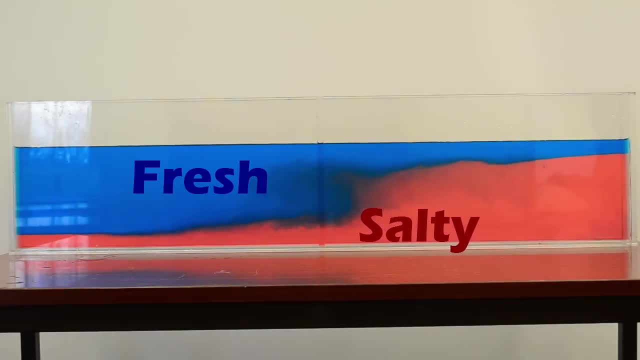 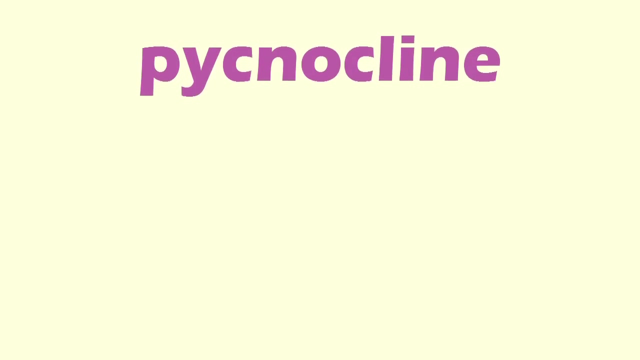 Since the salty water has a higher density, it sinks to the bottom. The same would happen if we had cold water on the left and warm water on the right side. Density differences have direct influence over ocean currents, pycnoclines, depth, among other properties. 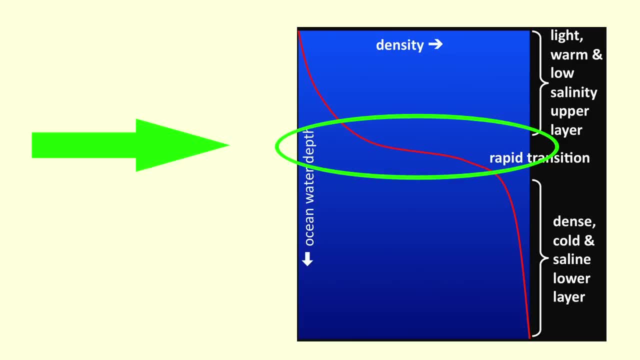 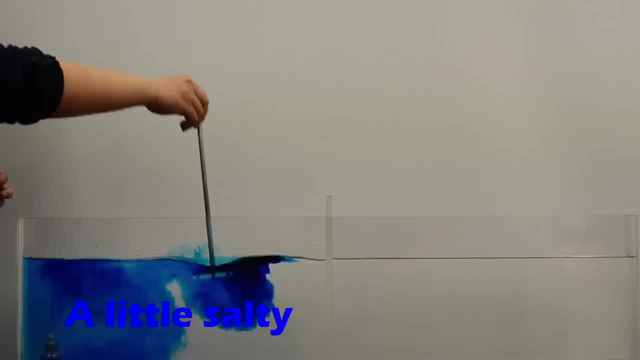 The pycnocline is the layer where the density gradient is the greatest within the ocean. In the second experiment, on the left side we have slightly salt water. On the right side there are saltier water on the bottom and fresh water on the top. 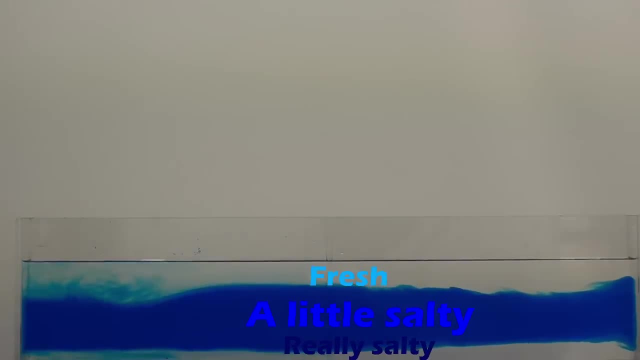 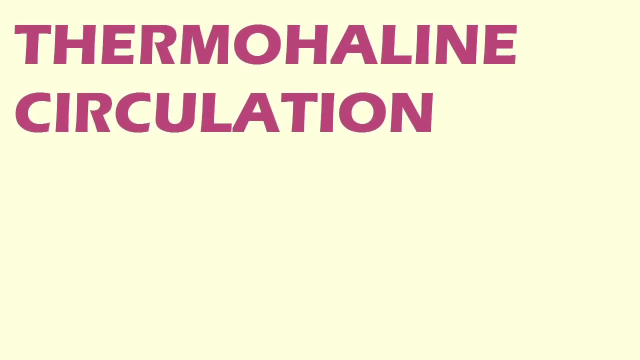 Since the water on the left has a density between pure and salty, it goes to the middle, showing the layer where the density gradient is the greatest. Finally, the water movement driven by density differences creates what we call thermohaline circulation. 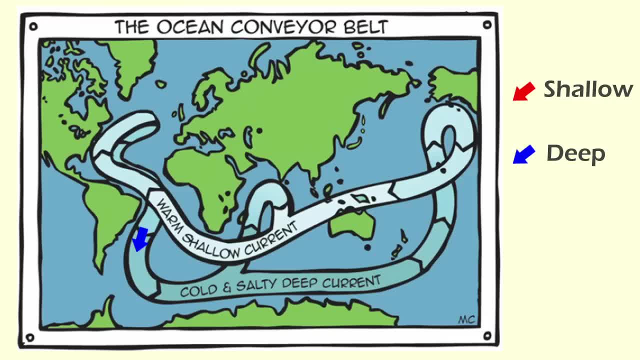 Thermohaline circulation moves a massive current of water around the globe from northern oceans to southern oceans and back again. Currents slowly turn over water in the entire ocean from top to bottom. It's somewhat like a giant conveyor belt, moving warm surface water downward and forcing cold waters upward. 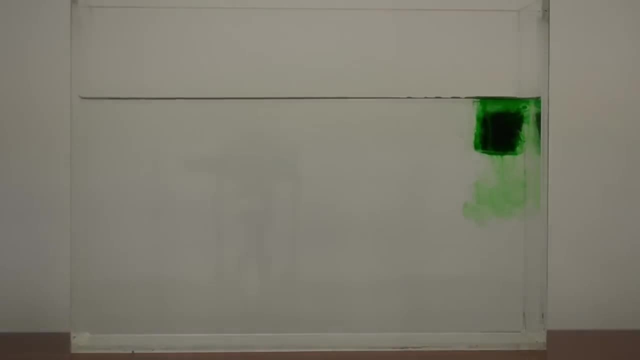 To help clarifying this concept, we added an ice cube on a tank with salt water. The melting ice creates the cold water that sinks to the bottom and travels to the left of the tank, similar to the waters that go from poles in the equatorial region. 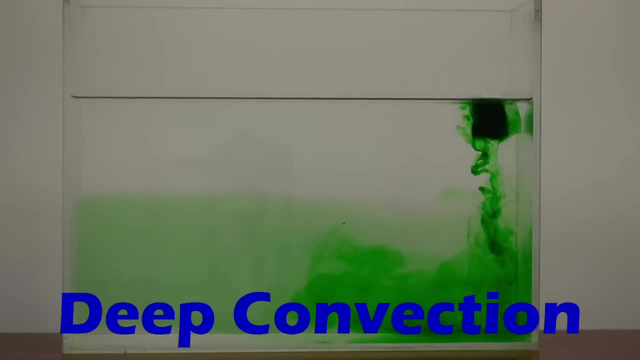 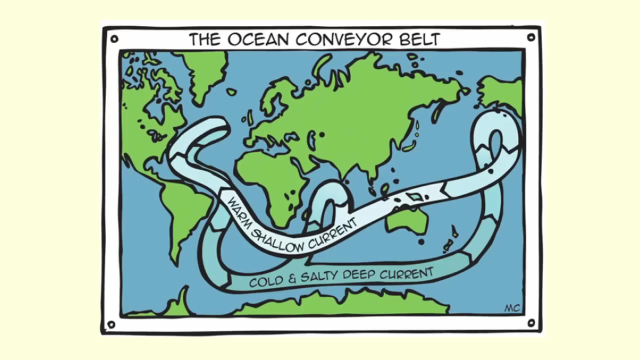 This is a process called deep convection, which is basically thermohaline circulation. This is the concept behind the Great Ocean Conveyor Belt, which is a constantly moving system of deep ocean circulation. However, this system can break down if the global temperature keeps increasing.